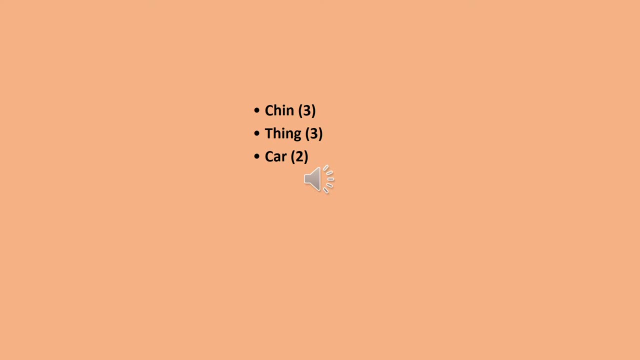 that CH sound. The word thing has three TH, A, N. You can't separate the N and the G and still get the N sound Again. a phoneme is the smallest unit that carries sound. CAR has two CAH with. 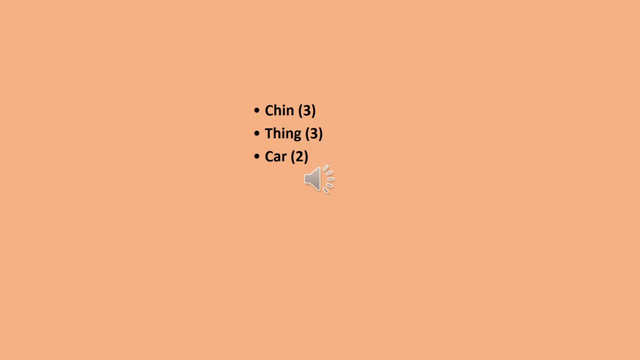 one and R would be the second. You cannot separate the A and the R and get the R sound. It would be K-A-R. A morpheme, on the other hand, is the smallest unit that carries meaning, So this could be a word like I meaning myself, or A meaning an object that carries meaning. 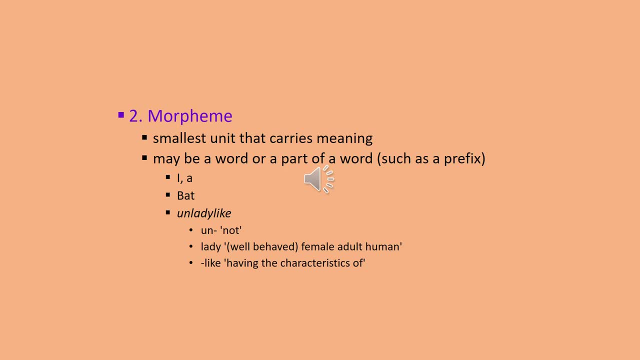 or it can be a whole word, like bat. You cannot separate that word and still have meaning. All prefixes and suffixes are also going to be a morpheme. For example, unladylike has a prefix and a suffix. Un- carries the meaning of not lady, a female, adult, human and like. 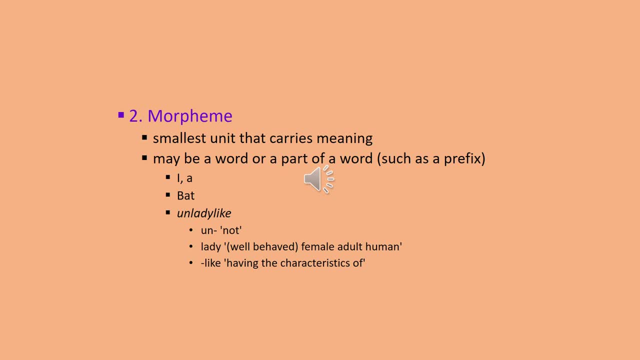 having characteristics of So unladylike would have three morphemes. Take a few minutes and number somewhere on a piece of paper from one to six and try and determine how many morphemes the following words would have in them: Number one: people. That would be one morpheme. You cannot separate that word and have meaning. 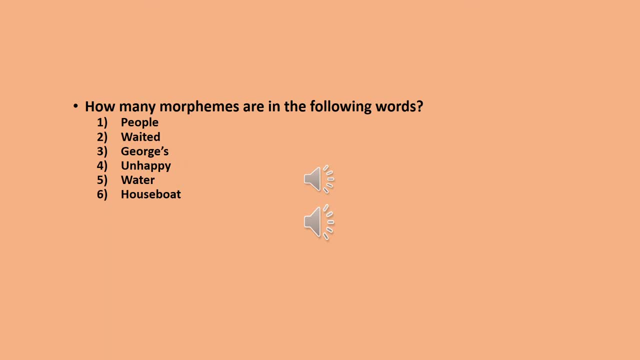 Number two: waited. That would have two morphemes. wait. and then adding the E-D makes it past tense. Georges, That would be two. You have George. and then when you add the apostrophe S, you make something possessive. 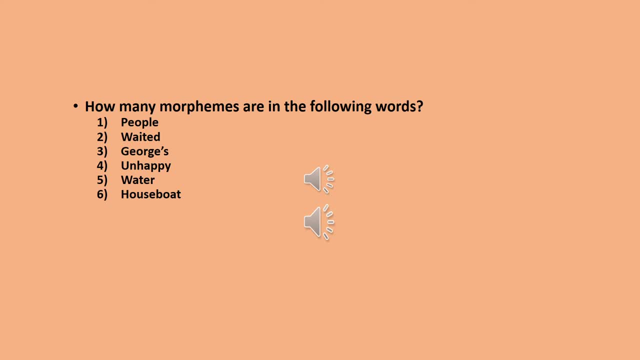 Number four has two unhappy un- meaning, not. Number five would have one morpheme. You cannot separate the word water and have any other meaning. Compound words will also be included with morphemes. Houseboat, for example, would have two morphemes: house and then boat.